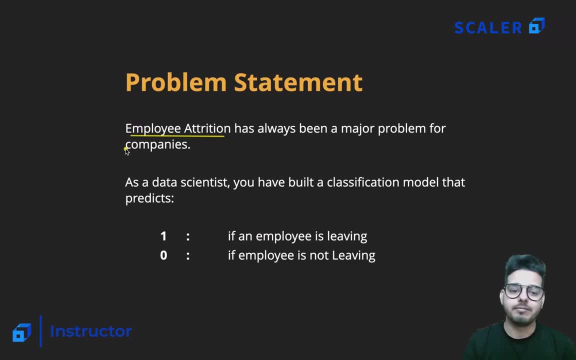 Okay, Maybe because of X, Y, Z reason, because of maybe another company is giving a higher salary, higher package, Maybe the employee thinks that the learnability curve in that other company would be higher, or maybe the workplace or the office is near to the new. 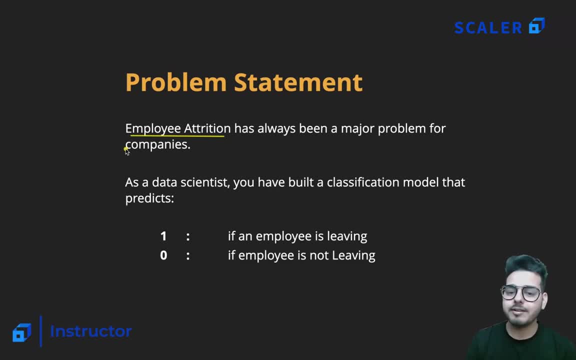 office that he is looking Because of X, Y, Z reason. if an employee decides that he wants to leave the company, so that would be a big problem for the current company because they would have to interview 10 different candidates for that one place. There would be a loss of some information. 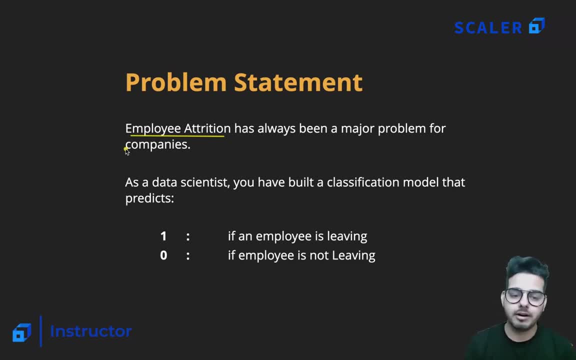 as well. right, So they would have to interview more candidates. All right, Now, as a data scientist, you have to solve this problem. Now, what you have done as a data scientist? you have built a classification model, Okay, That can predict if an employee is leaving. 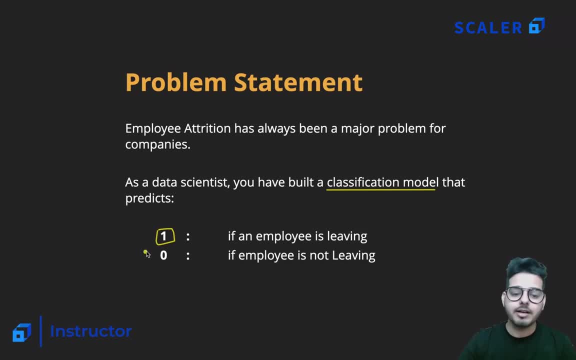 it will predict one, And if the employee is not leaving, it will predict zero. Okay, Why do we call it as a classification model? Because it is categorizing. It is categorizing into two categories. For example, if employee is leaving, it will say one, Yes, employee. 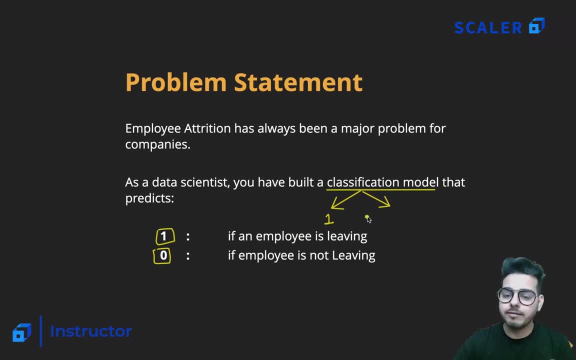 is going to leave. It will predict employee is going to leave and zero if the employee is not going to leave. That's why it's called the classification model. So in this video, how to build this classification model- you can check out other videos on the intuition. 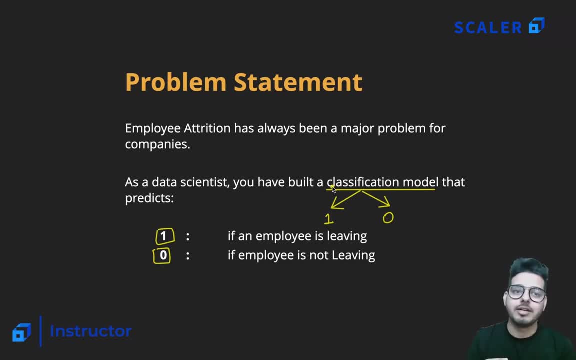 of logistic regression, intuition on decision tree, So there can be multiple classification models that you can use. For example, logistic regression is one model, one such model that you can use. Decision trees can be another model that you can use. Okay, So in this video, 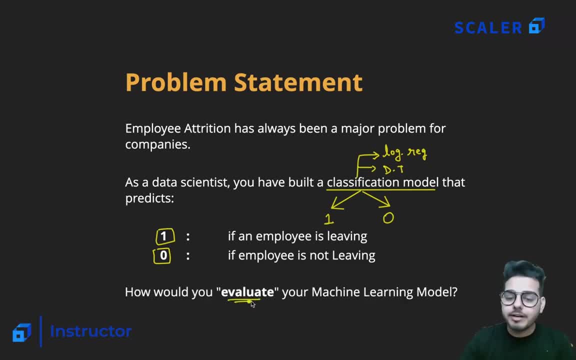 we will be talking about how to evaluate your machine learning model. You have built the machine learning model. You have built the machine learning model. You have built the machine learning model and it's working fine. It is predicting for an employee If you provide. 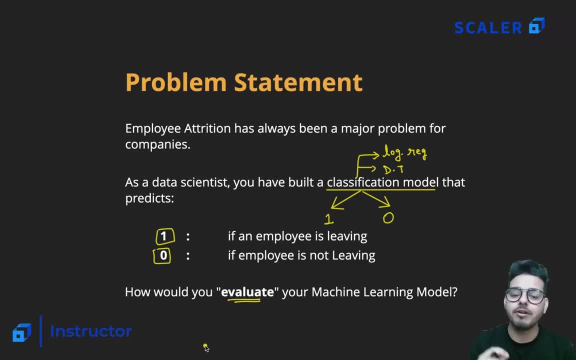 an input to the model. it can predict the employee is going to leave or not, right, Not leaving, So it will just predict one and zero. Now the important question is that we have to solve, We are solving in this video is: how would you evaluate that? the model that? 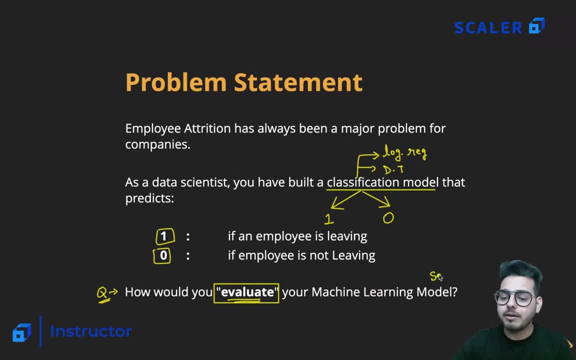 you have created is sensible. This would be an important question to ask Why it's an important question Because, Hey, I can create a machine learning model. I can create a machine, create a model that can predict all 11111 for all the employees. It means that I'm saying Hey, 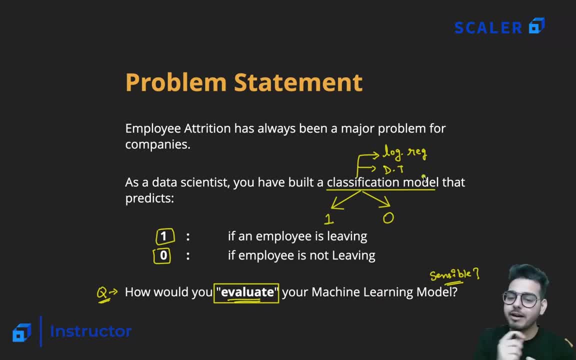 this employee is leaving, Second employee is also leaving, Third employee is also leaving, and all the employees are leaving. This is not a sensible model, right? Or in other case, I can just say, Hey, no one is going to leave, Just predict 00000 for everyone. Again, this is not a sensible model. 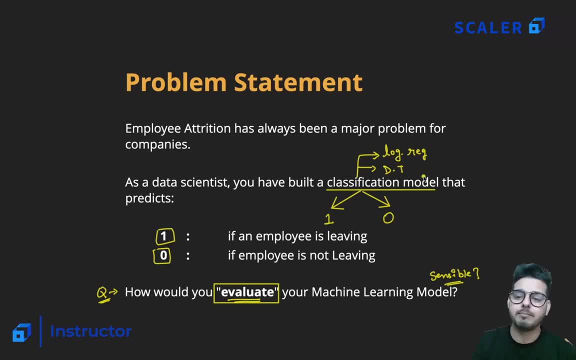 So to put any model in the production, before putting any model into production, I need to evaluate how good the model is going to be in the production. I need to evaluate how good the model is, how sensible the model is, how sensible these predictions are from this particular model Or 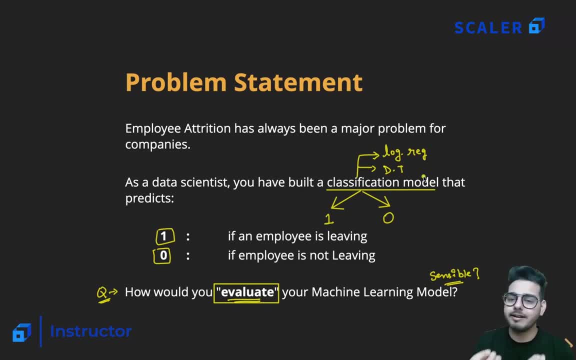 even sometime, if you have five different models. let's say, in our data science, data science team we have created five different models. Now which model to put in production? we can evaluate all the five models using confusion metrics And then the best model. 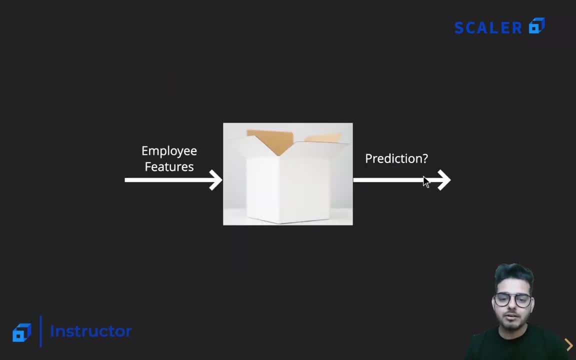 we can put it in production, All right. So what we have is something like this: We have a model, machine learning model, Okay, It can be logistic regression, It can be decision tree, It can be SVM, any model. What I'm concerned about, Okay, This: I'll provide the employee features, I'll 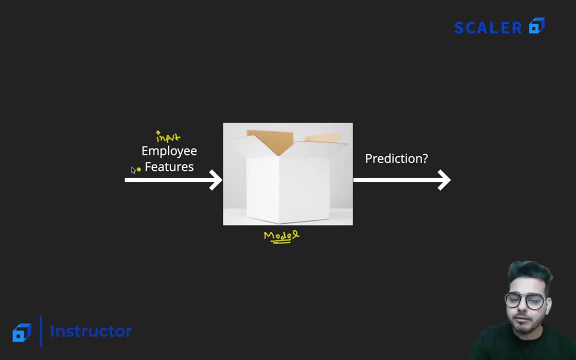 provide this as input. What are the features? Features can be: what is the current salary of the employee, How, for how many years this employee is working, Maybe the work experience Okay, And what is the team He works for, and so on, so forth- The other other features that you have for an employee. 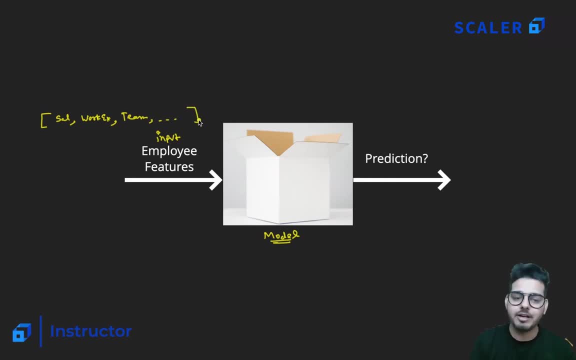 how you, how you represent an employee right. So if you put all these features as input, this is for one employee, Okay. Similarly, if you input another employee, features of another employee right, This model will give you the prediction It can give you. 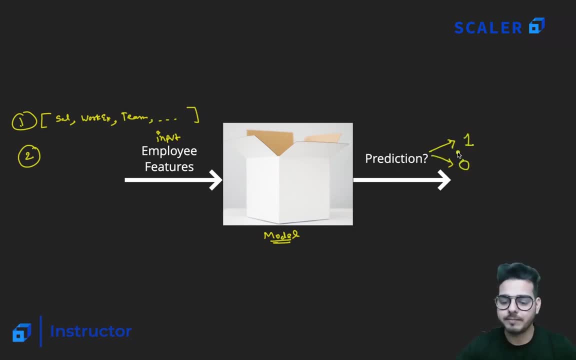 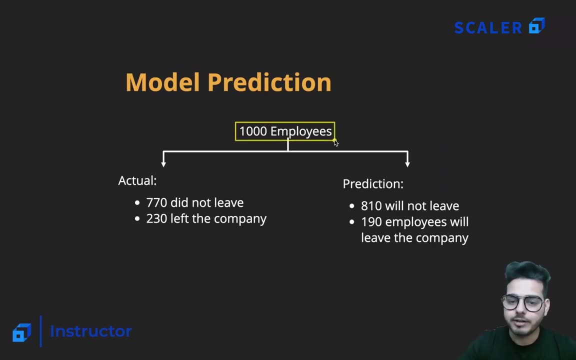 whether the employee is going to leave or not leaving. So this is what we have. Okay, Now let's understand. let's say there are hundred thousand employees in a company and the actual data says that 770 people did not leave the company in the next month, And out of thousand, 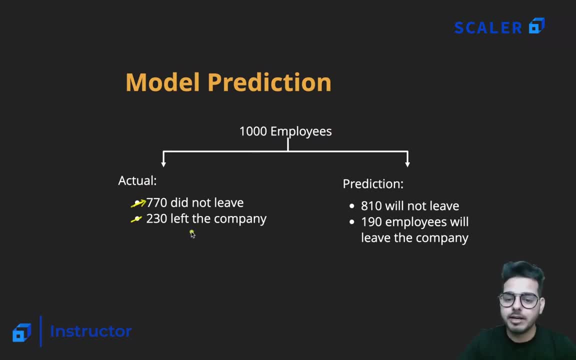 people, 230 people- left the company. Okay, But when, if you, if you input these thousand employees to your machine learning model, the machine learning model says that 800 people will not leave the company, Okay, month, let's say, since we are predicting for the next month only, uh, let's say, 800 people did not. 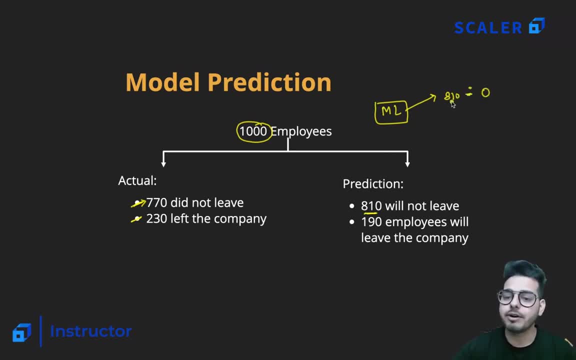 leave, so it is predicting zero. it is predicting zero for 810 people and for 190 people it is predicting category one. okay, this is the predictions you have from your machine learning model and, in actual, what we have observed is 770 people did not leave, whereas 230 people left the company. 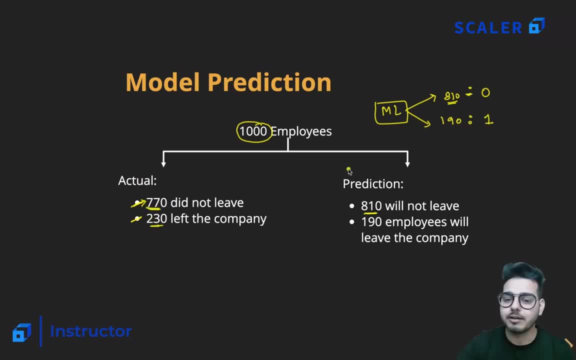 now i need to understand: is this model, the model that we have used here, is a sensible model or not? is it a sensible model? because you can see that there are some misclassification, right, but i want to understand in more depth, and that's why we will. 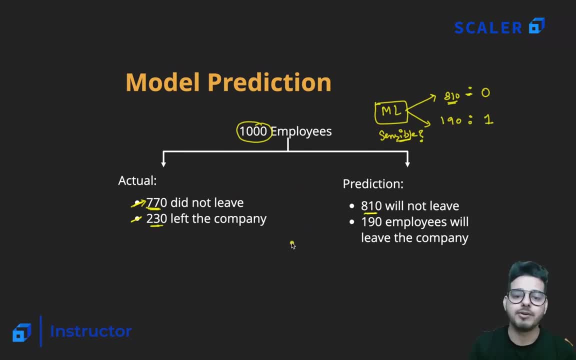 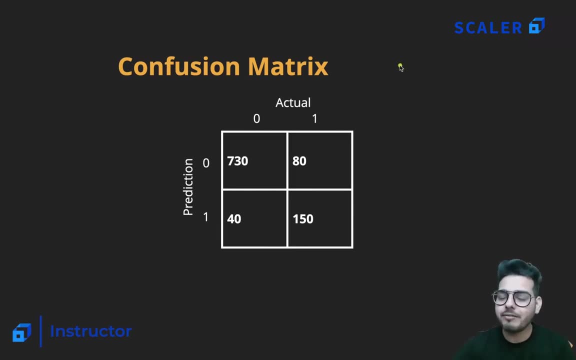 understand the confusion matrix and we will plot the confusion matrix. so the confusion matrix is actually a matrix. so, for example, if you have two categories right now, one is the confusion matrix and the other is the confusion matrix. so for example, if you have two- have employee will leave or will not leave, i have two categories. so the matrix that i will plot, 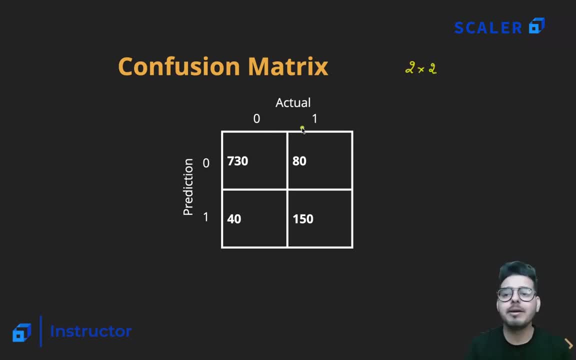 will be two cross two. if you have three categories, maybe in any differentiation or a different challenge you can have three different categories. in that case the confusion matrix would be three cross three. if you have four categories, four cross four. if you have k categories- k is a general term- 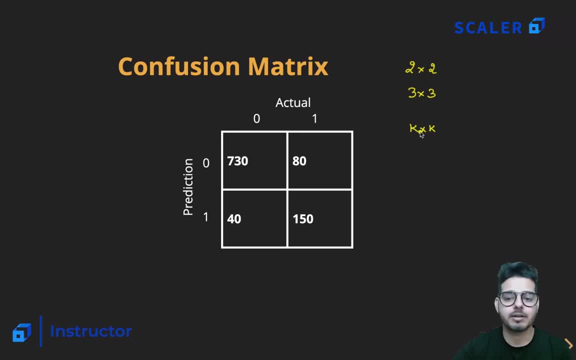 then the matrix that you will plot would be k cross k. okay now, since in this problem that we are tackling right now, the, the, there are two different classes, let's stick to only two cross two matrix. so this is how the confusion matrix look like. on this on the column side, we plot or we put the actual labels, actual categories. what are the actual? 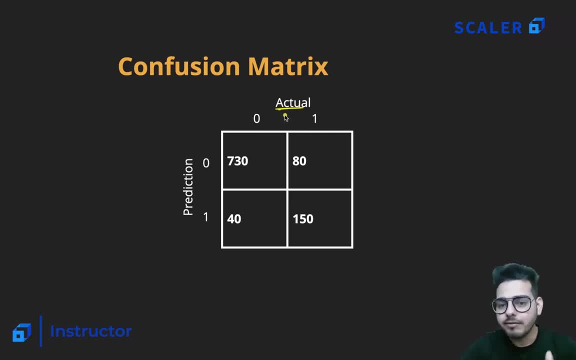 categories. the actual categories were: employee will leave one. employee will not leave zero, so employee will leave it's one. employee will not leave it's zero. on the rows side, on rows, we will put predictions. now. predictions can also be zero if the employee, if the model says that employee is. 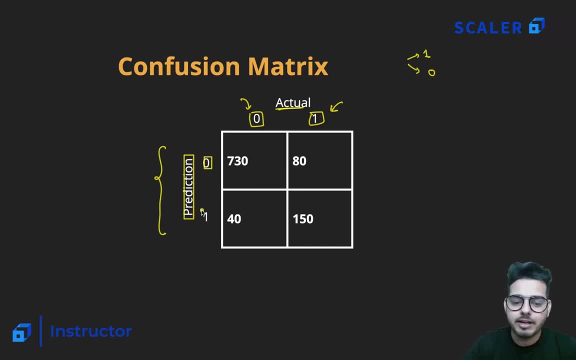 not going to leave and one if model says that employee is going to leave, okay, and hence it. this look like a grid. okay, this look like a grid. so what we observed is that the model says that the employee is going to leave and the company is going to leave. so what we observed from the data, 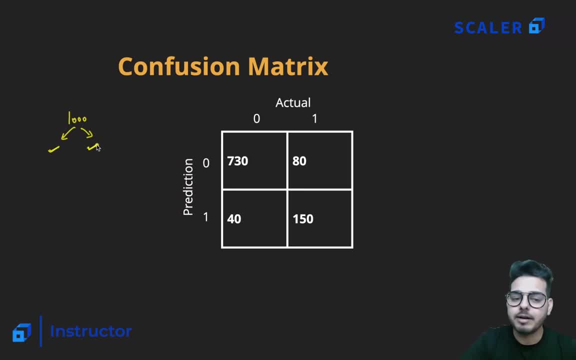 is for thousand people. we had thousand people model said that, okay, few people will leave, few people will not leave, but in actual, we saw that, okay, these number of people left the company and these number of people did not leave the company. okay, so let's understand and let's plot the data. 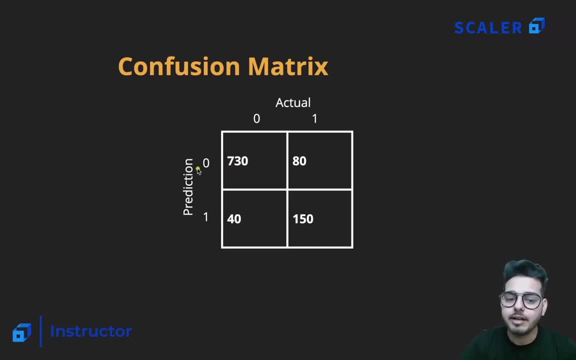 uh, in the confusion matrix, so it looks something like this: so this number 730, it says that, hey, your is saying that these number of people will not leave the company. that's why it's zero. zero means will not leave. in actual what we observed, that they didn't leave the company. and this is the 730. 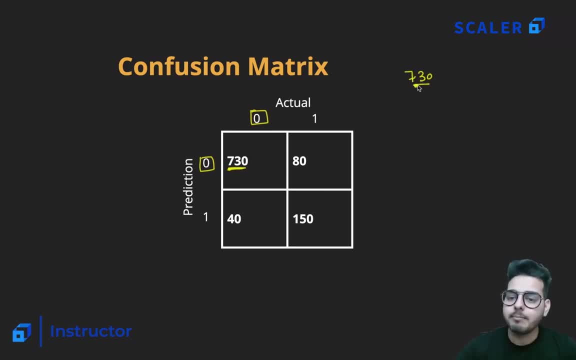 so these 730 people or employees, model said that they will not leave the company in the next month and in actual they didn't leave, right? so it means the model is correct about these 730 people. so out of thousand at least, model is correct about these 730. 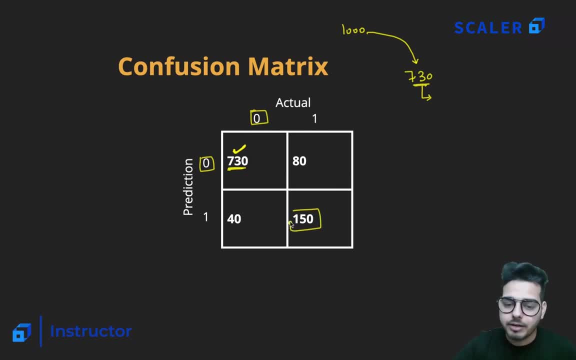 people or employee. look at these 150. what exactly this 150, uh, is saying so? this 150 is saying that the prediction is one. prediction is one means. model is saying they will leave. right model is saying that these people will leave and, in actual, we observed that the next month they. 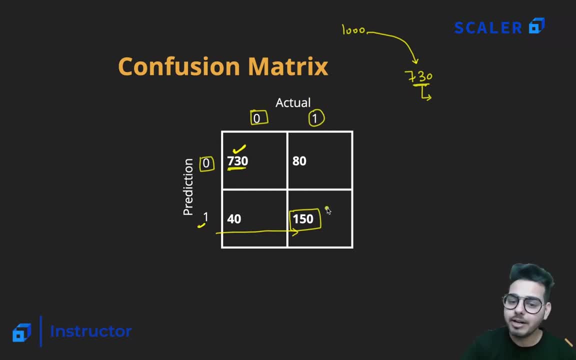 leave or they left the company. so it means again, model is correct about these 150 people. model is correct about 150 people, right? so out of thousand people, i can see that, okay, these 730 people plus 150 people. model is correct about these number of employees. but what about this 40 and 80? what about this 40? 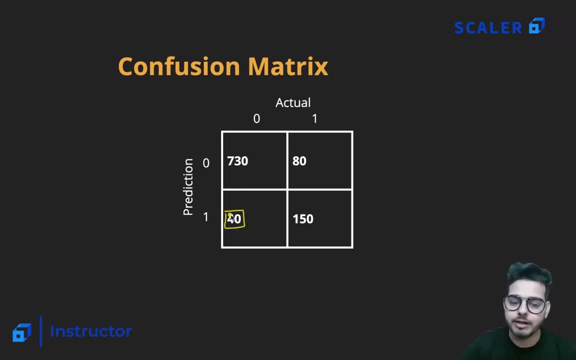 entity. let's understand this term 40 right what exactly this number representing the model is. presenting model is saying that these employee are going to leave, but in actual, what we observed is that they are going to leave. so, for example, if someone who is happy with his job, well settled. 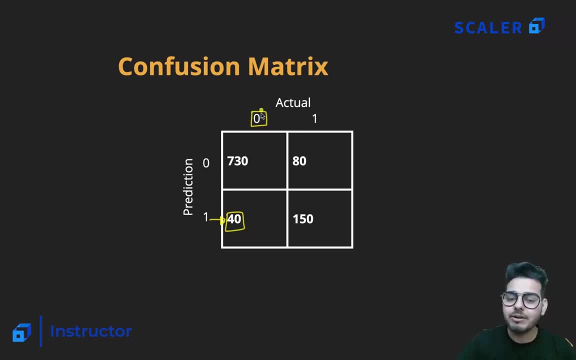 and so he's happy with the job, right? he will not leave the company. why would he leave the company? but your model is saying that, hey, this person is going to leave in the next month, which is wrong. which is wrong, right? similarly, look at this one 80 model is saying that: 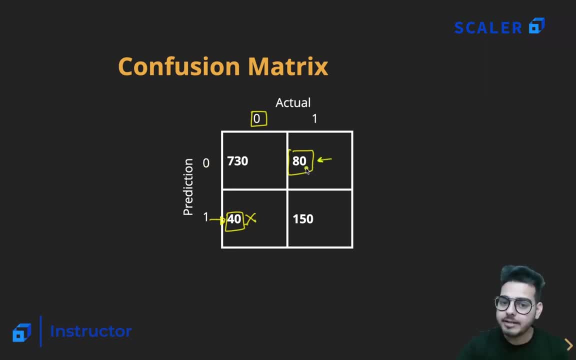 this: these 80 people are not going to leave, whereas in actual, what we observed is they left the company in the next month, which is again model is wrong about these 80 people. so 40 plus 80. the model is giving wrong prediction for 120 employees and for 880 people, or 880 employee. 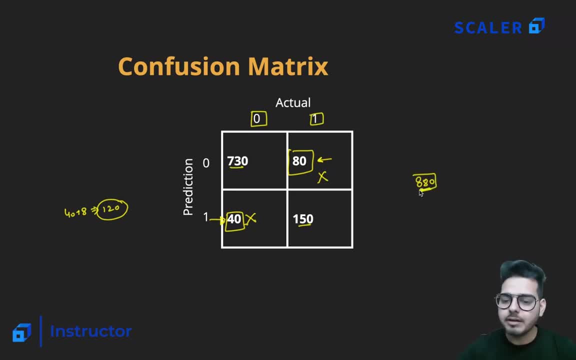 730 plus 150 for 880 people employees model is giving the right prediction, correct prediction and hence we can say the accuracy of a model is 880 divided by 80.. thousand, that will become 88. okay, so it means that 88 accurate. we have the accuracy of a model. 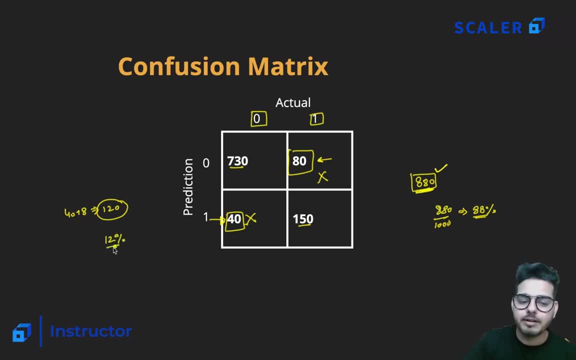 80 and the error would be 12. okay, let's give the terminology to the confusion: matrix. so this thing, uh, so we can see that over here we have tn, then fn, fp, tp. let's understand what exactly this tnt and tp, fp is, so uh. 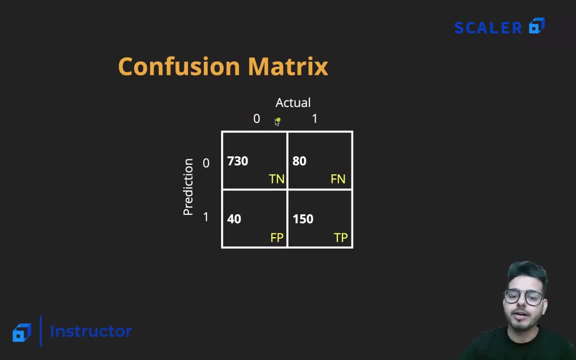 in the machine learning terminology when we have two categories, zero and one, generally zero category is termed as negative category or negative class. okay, or negative category or label, you can say. one is generally called as positive category or positive class. so if you sum across this column, you will. 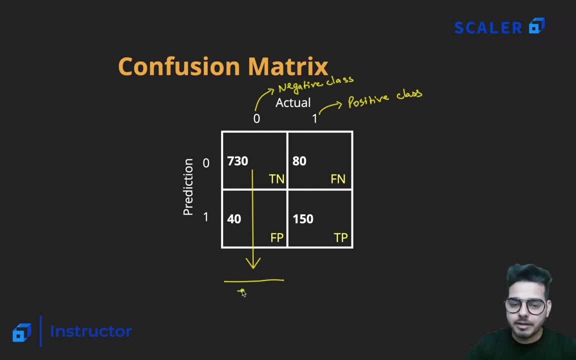 get seven, thirty plus forty, that will become uh, seven, seventy, okay, and if you sum across this column, this will become 80 plus 150, 230. so it means in actual, in actual, there were 770 negative people. negative people as in they did not leave. in actual and in actual, there were 230 positive. 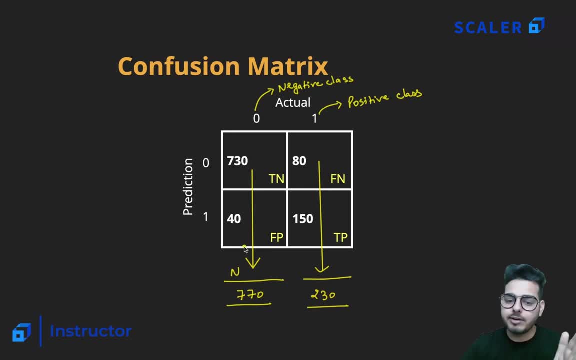 people. so this is the total negative- total negative in actual data and this is total positive in the actual data: 230 people actually left. if you sum across rows, this will be the prediction of zero, right? so this is 730 plus 80. this will be 810. model said that 810 people will not leave the. 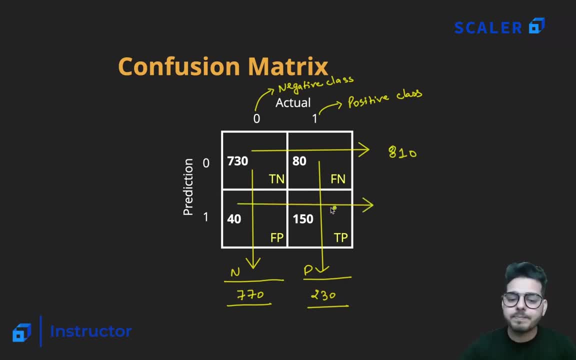 company and if you sum across this row, this would be 40 plus 150. this would be 190. model is saying that 190 employee will leave the company. okay, so this is np negative, positive and this is the prediction of the negative class. this is the prediction of the positive class. now let's 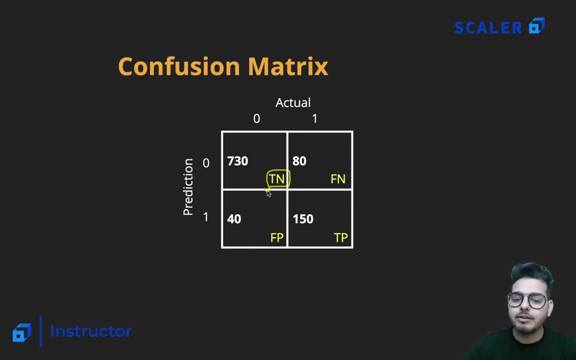 understand about this terminology. what is this tn? so this tn? there are two terms. there are two terms over here. the first is what your prediction is from the model, what the model is predicting now. in this case, model is predicting class 0, and class 0 is termed as negative. so i will write n. so, by the way, negative and positive. 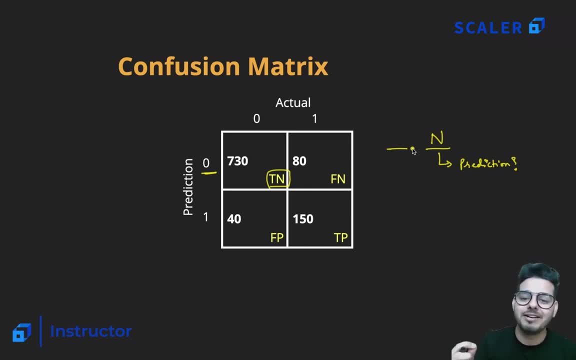 so positive. the term positive is not coming from a positive news. so here in this, in this case, when the model is saying 1, 1 means positive. right, but this is not a positive news for the company if employee is leaving. but this is general terminology and don't relate this positive with a positive news. positive is just because one and 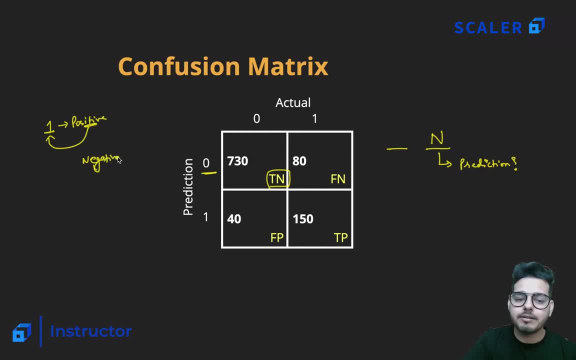 negative would be. negative would be because it is zero. okay, because this is zero, all right. so this first. i need to put n. why? because model is predicting zero and zero means negative. now this second term would be: is my model correct? is model correct in the prediction? whatever the model model, 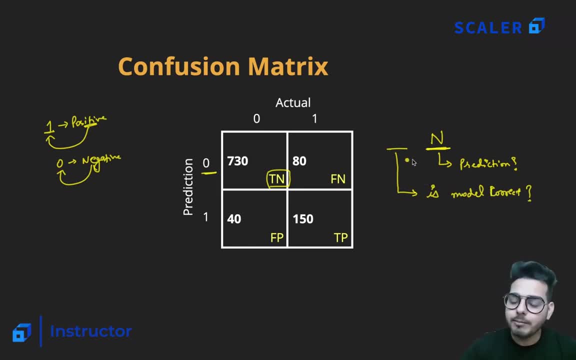 has predicted, is model correct in that prediction. so if the model is correct, then it means i need to put true and yes. in actual it is zero. model also predicted zero. it means this is true. model is saying true right, so that's why it's called true, negative. let's look at this term: it's tp right, tp so. 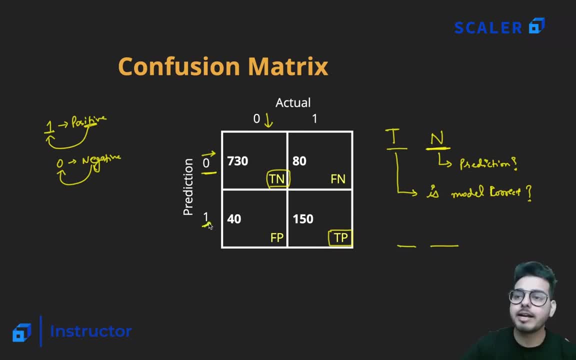 what model is predicting? model is predicting class one, category one which is positive. this is the prediction right. this is the prediction from the model. now, is my model correct? yes, because model predicted class one and in actual it's also class one. it means model predicted that these 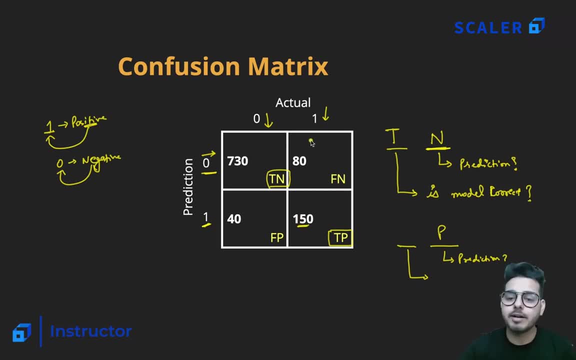 people are going to leave and, in actual, these employees left the company. that's why it's true, true, positive. look at this one right. look at this one right. look at this one right. look at this one. look at this fp, fp, right. what your model is predicting model is predicting that these people 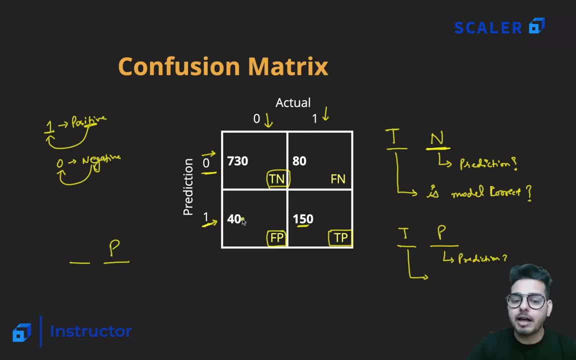 are going to leave. that's why positive: class one, right class one. but is this model correct? no, in actual, they did not leave, these employees did not leave and that's why it's false. it is kind of it we call it as false positive. it is kind of false alarm. you are saying that. 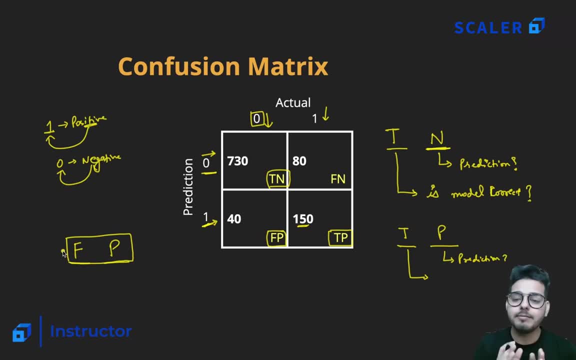 hey, these 40 employees are going to leave. right, these people are going to leave, but in actual, they're not leaving, they're happy with the job. so you will be putting a lot of extra resources um for for retaining these employees right, and that's why it's called false. 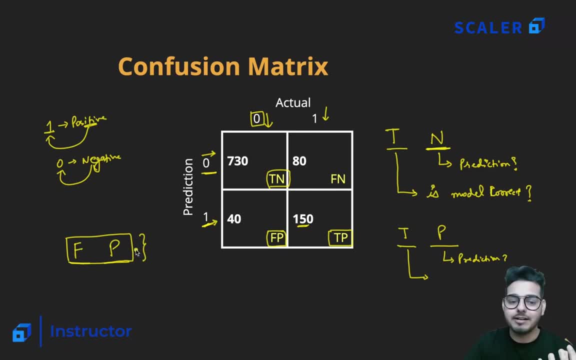 alarm you're. you're generating an alarm that hey, uh, make sure that these employees will not leave. but they're not leaving. they're not leaving, right, they're happy with the job. that's why they're called as false positive. look at this one. this is false negative. what you are predicting class. 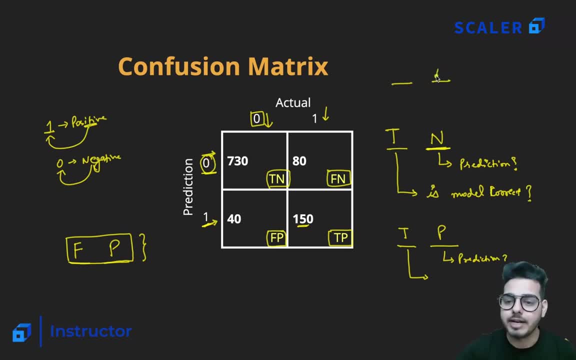 zero, they will not leave. you're saying employee will not leave, negative, all right, but in actual they left the company. it means you're telling wrong. right, the model is predicting wrong, so that's why it's false and this is the most critical number, why your model is saying that. 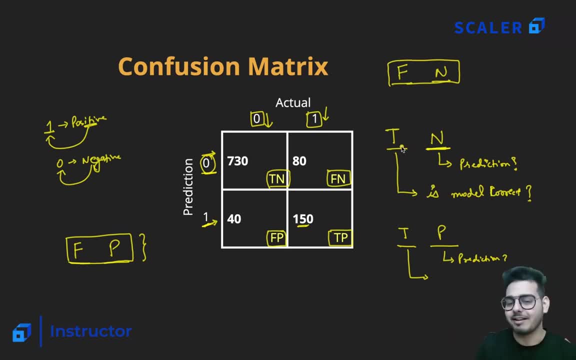 hey, these employees are not going to leave, so be relaxed. relaxed, right, but in actual they left the company. in actual, they left the company and we wanted to retain these employees. that's what the purpose of the machine learning model is, right, that identify those customer, those employees who 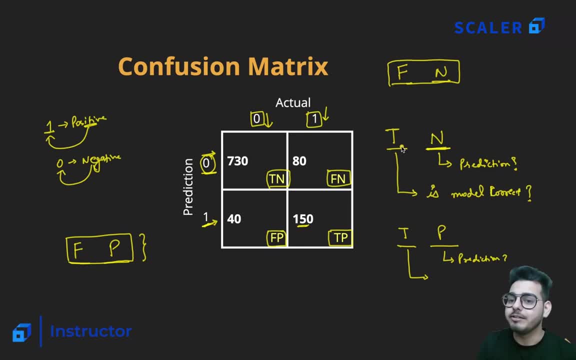 are going to leave and retain them so that we can put energy resources in retaining them, but the model is not able to predict. model is saying that, hey, these people are not going to leave, which is wrong, and hence this would be very, very important number. i want this number to be very low, ideally. 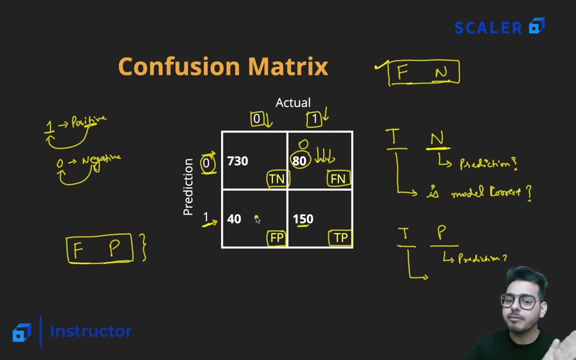 it should be zero, that no employee is left, like if the employee in actual is leaving, then the model is not predicting wrong model is not predicting that he is not uh, leaving right. so ideally, these two numbers, false predictions, false positive and false negative. ideally they should be very low. ideally they should be zero. ideally it should be. 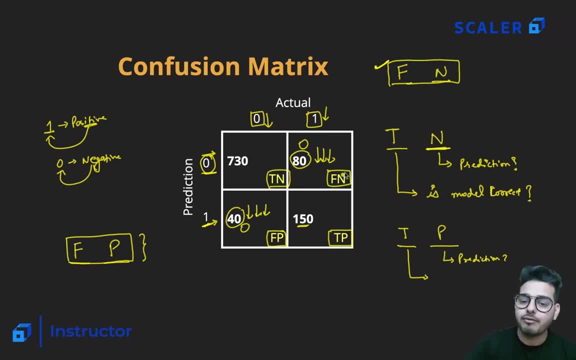 zero. but we should have a model having false positive and false negative to be as low as possible, and these two numbers, tn and tp. so always remember the diagonal element should be very high, the diagonal element should be high and the of element, the rest of the element, should be very low. then i will say that my model is: 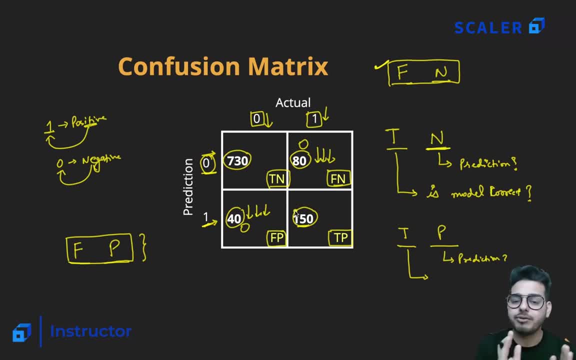 sensible. so if you want to compare two models, just plot the confusion matrix for these two models and observe these false positive, false negative, true negative, true positive. the diagonal elements should be higher. and if you are concerned about these employees for exampl, these are the employees, are those employees? the model predicted that these are not leaving, but in actual they left. 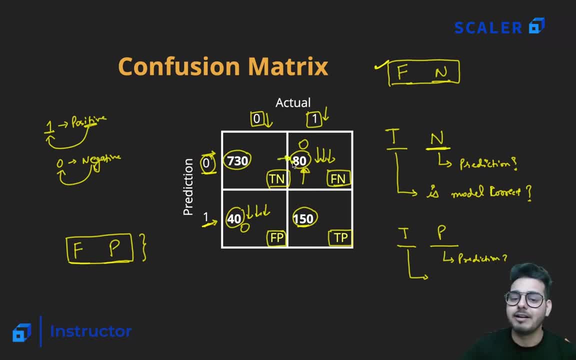 so this is the most critical number. i want this number to be as low as possible. right, and that's how we can plot the confusion matrix. we can evaluate a machine learning model, and the accuracy of this model would be: tn plus tp divided by all the numbers, divided by tn plus tp plus fp plus.